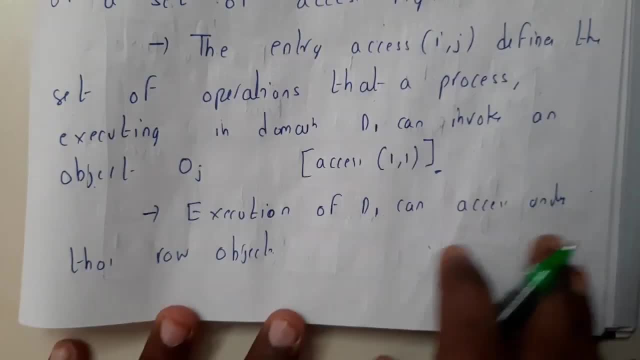 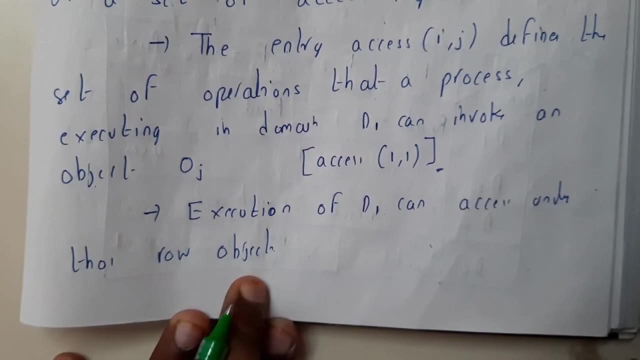 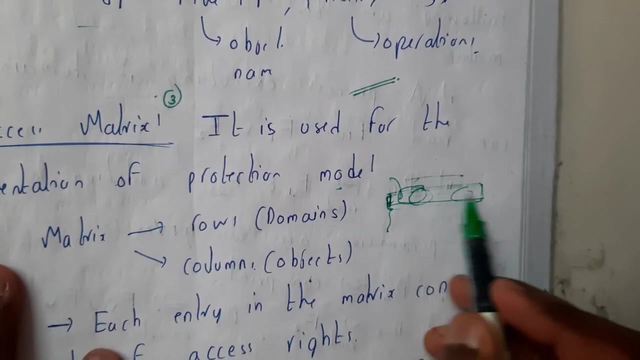 first file, its access rights will be printed or it will be collected in that way. So execute D1 can access only the row objects. If I write access execute D1, it is going to print this whole row guys row or column, row data. 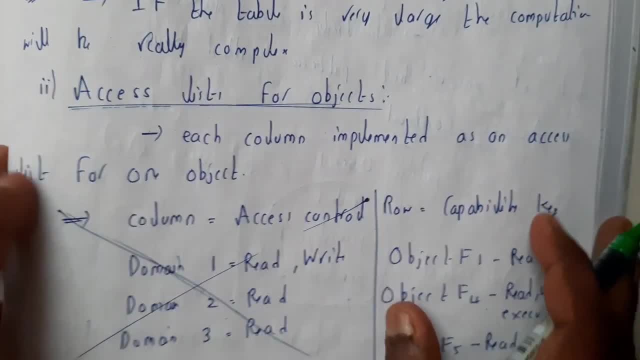 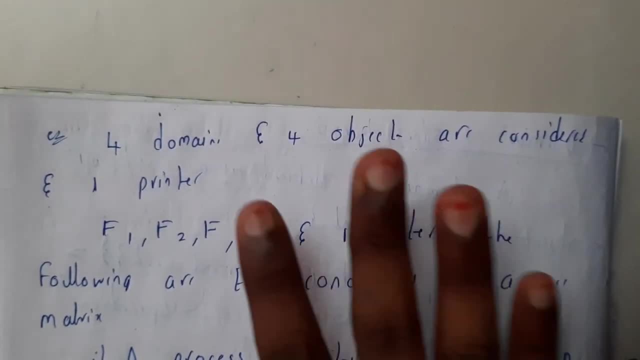 Whatever file it might be, it will be printing the whole row. So once we are going through the example, you will be having a clear idea, guys, don't worry. So here there is a small question which is given. He told that there are four domains and four objects and one printer. So 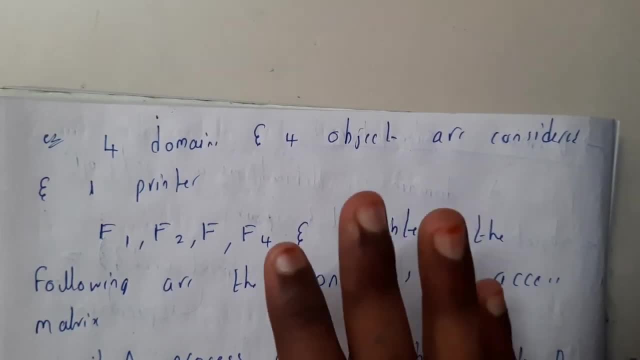 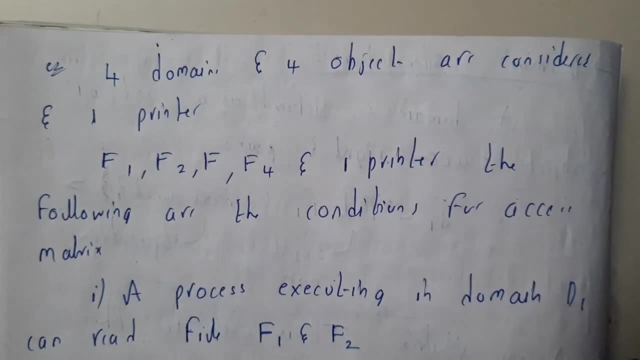 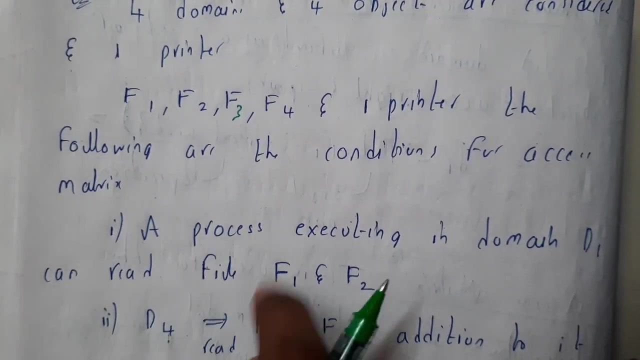 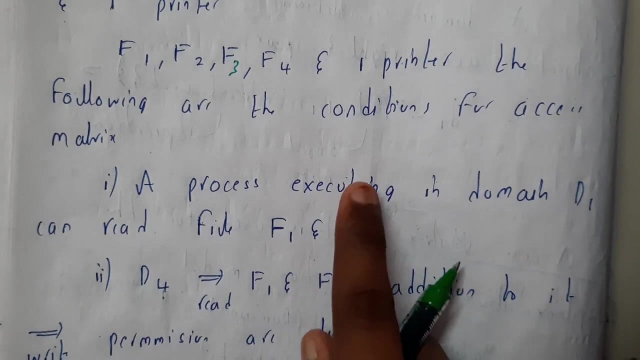 there are totally five objects and four domains. Fine, So the four objects given are file 1, file 2, file 3 and file 4, and one printer. The following are the conditions for the access matrix. So they give you conditions. A process executing in domain D1 can read file F1 and F2.. Once I'll be 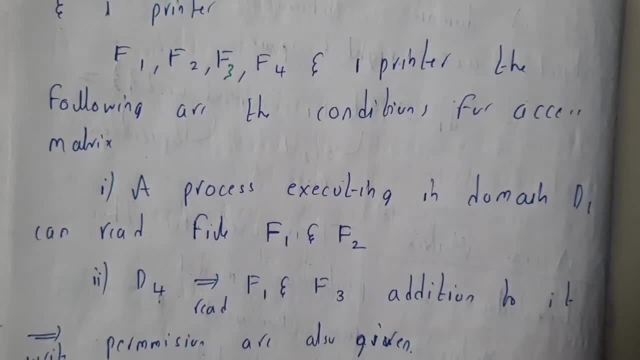 reading these all things, guys. after that we will be solving. So you also take a small piece of paper and you solve with me so that it will be clear for you. A process executing in domain D1 can read file F1 and F2.. 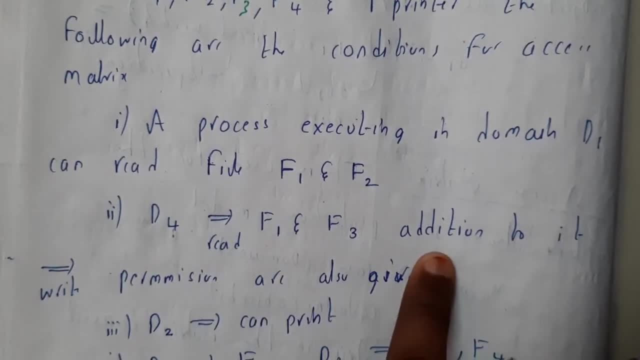 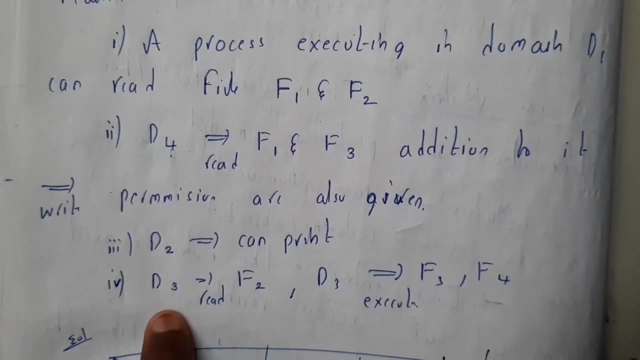 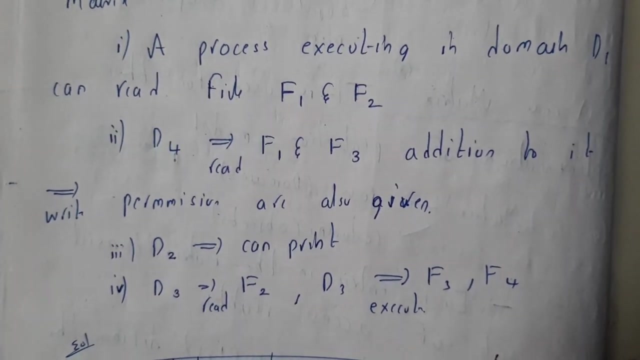 D4 can read F1 and F3.. Edition 2, it can also write in F3.. D2 can print: D3 reads F2.. D3 executes F3 and F4.. So these are the things which are given, So let us now try to draw the access matrix for this. Guys, this topic. 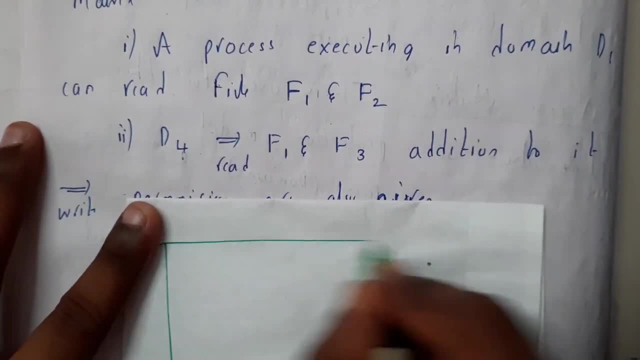 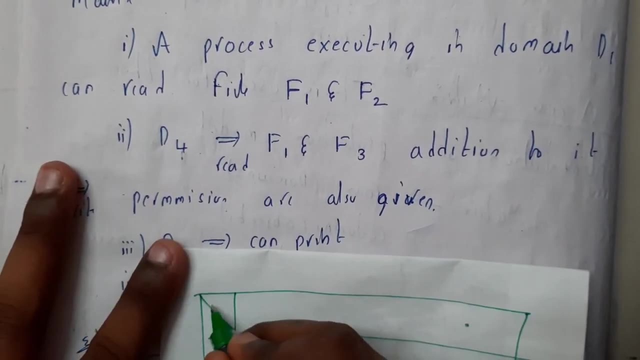 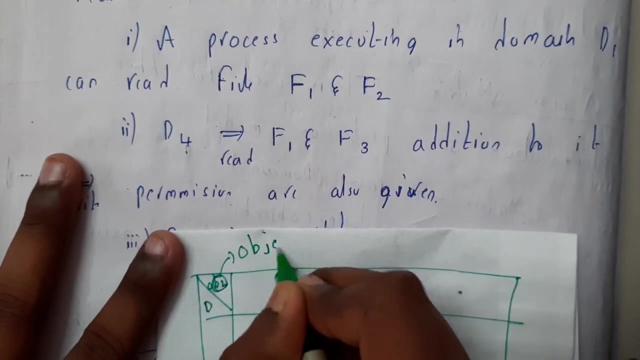 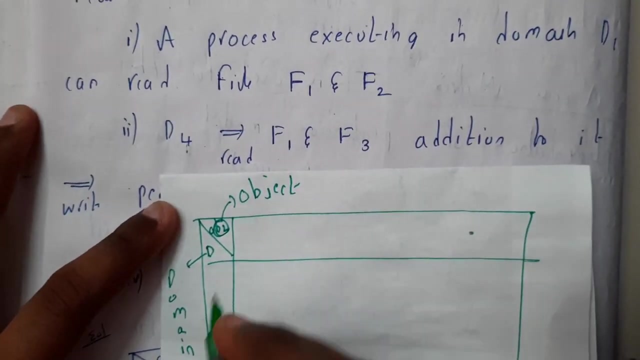 is really simple, guys. The thing is that you should understand the concept. So above we'll be taking objects and below we'll be taking objects. So above we'll be taking objects and below we'll be taking domains. I'll be using a single letter: O means object, D means domain. Fine, Okay, So from the 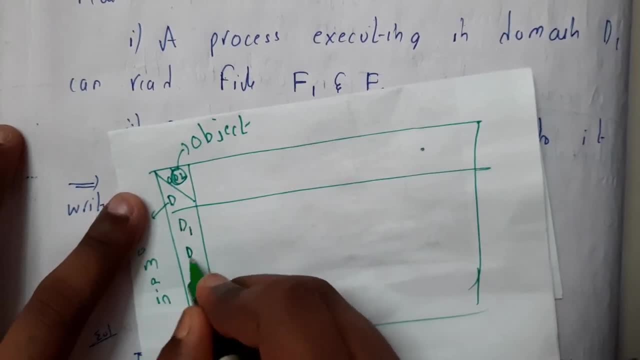 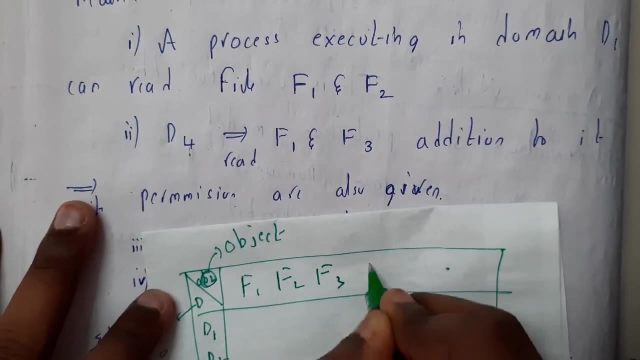 question that he gave four domains, So let me give the names as D1, D2, D3, D4.. Mainly he will be giving these names in the question itself, guys, So please concentrate while you are reading the question. F4. and he also told about the printer.